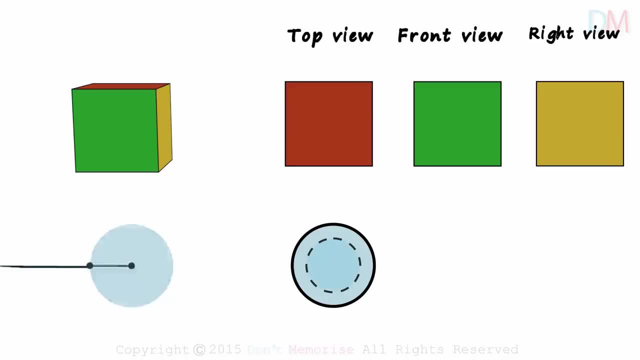 And if the top wasn't covered, we would see the circle of the base as well. And what about the front view? Pause the video and give it a thought. This is what we would see: A trapezium, Two sides parallel and two non-parallel. 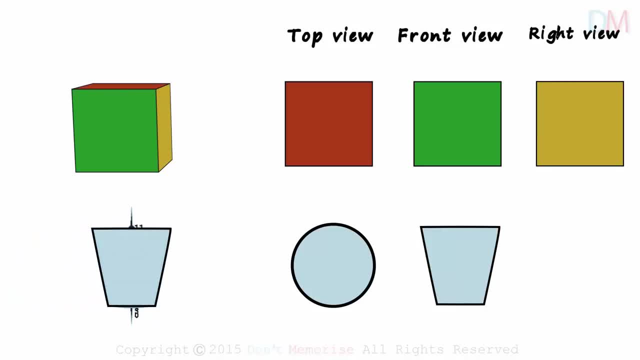 And the view from the right Again, it would be a trapezium. No matter which side you look at it from, we will always see a trapezium. So imagining the views was pretty easy here. How about we make it a bit more exciting? 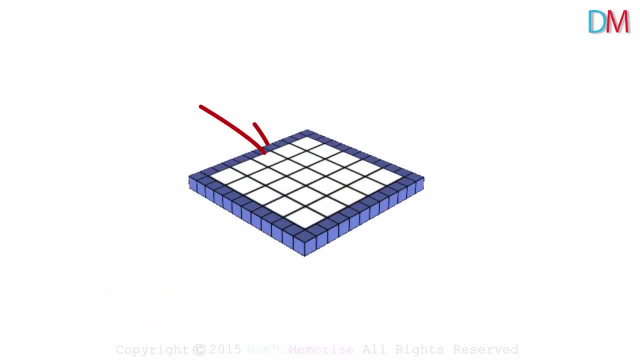 I will be placing a square here. I will be placing a few coloured cubes on this plain surface to form a figure. Okay, so here it goes. I place two red cubes here, one yellow cube on top and one blue cube here. This is the solid we will be referring to for this example. 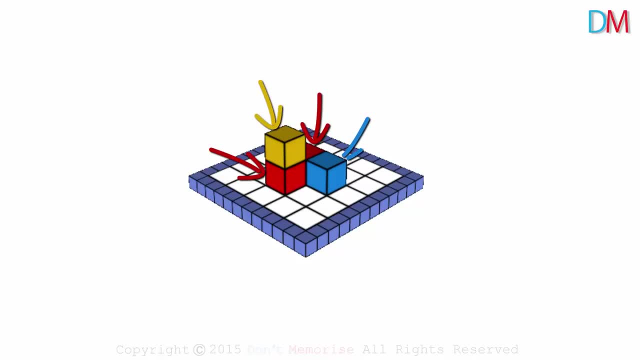 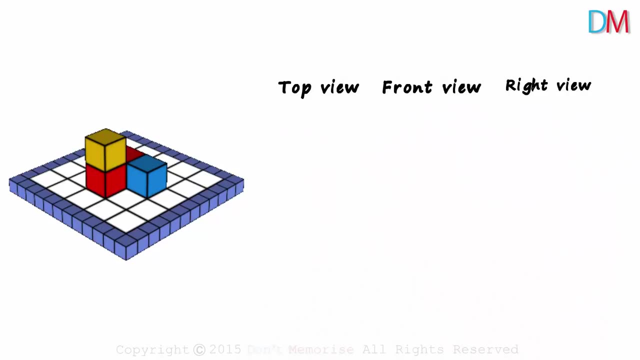 We have two red cubes, one yellow cube and a blue one. Now we need to draw the top view, the view from the front and the view from the right. How would the top view look? Pause the video and try to draw it in your notebook. 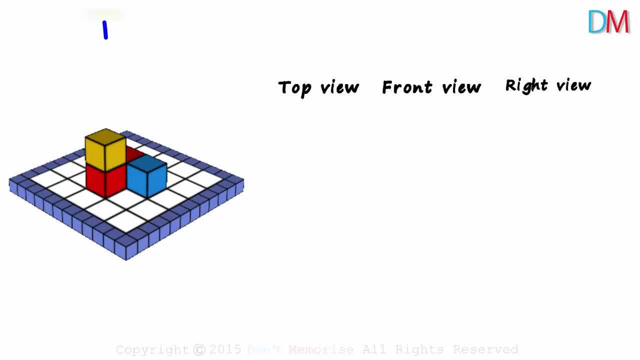 Let's try drawing it without moving the figure. If we look at it from the top, we will have the yellow square at the bottom. We draw a yellow square here And this red cube will not be seen from the top as the yellow one is covering it. 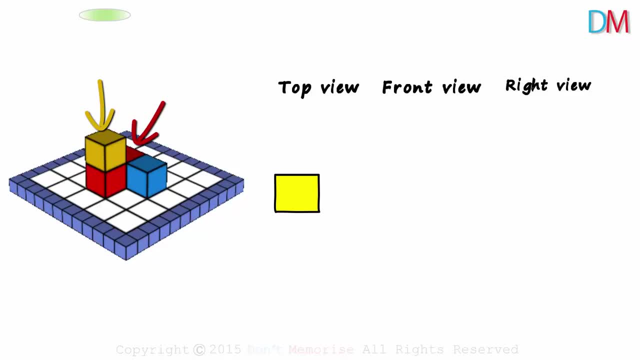 Next to the yellow square we have the top face of the red cube, So we draw the red square face here. And to the right of the top face of the red cube we have the top face of the blue cube, So we draw a blue square here. 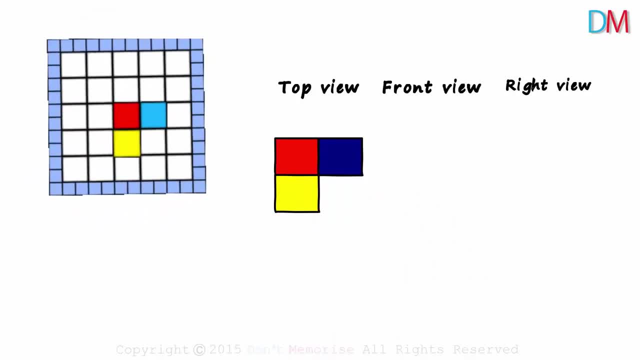 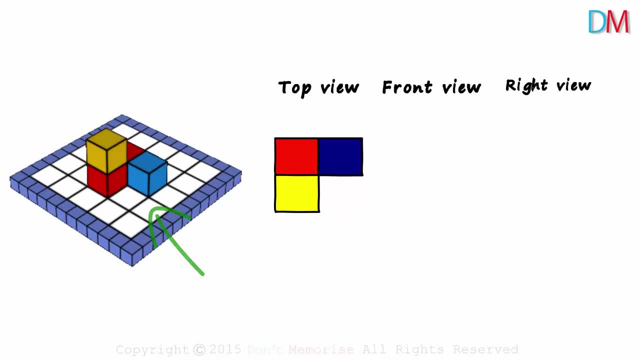 This will be the top view. If we take the camera on top, we can see that our figure is correct. Now let's get back to the original view. Looking at this, I want you to try drawing the view from the front and the view from. 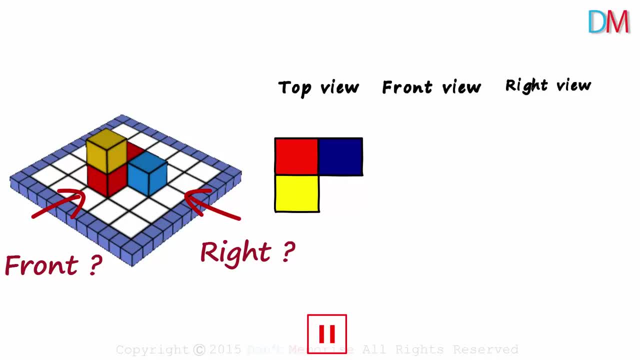 the right. Okay, let's see. Ok, let's draw the front view first. The front view is the view from here. At the bottom we have the front face of this red cube. So we draw a red square here. Imagine you are standing here. 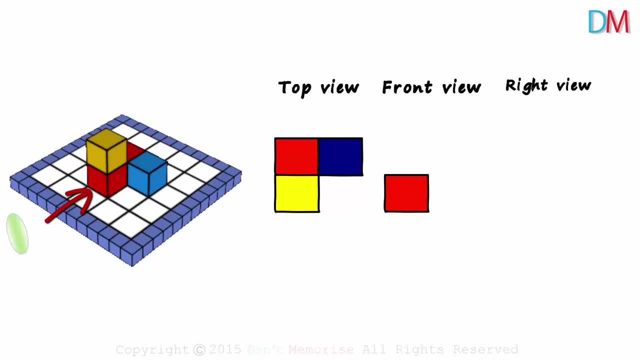 Now, from the front view, what will we see on the top of the red cube? It will be the front face of the yellow cube. So we draw a yellow square on top of the red one And at the bottom, next to the front face of the red cube. 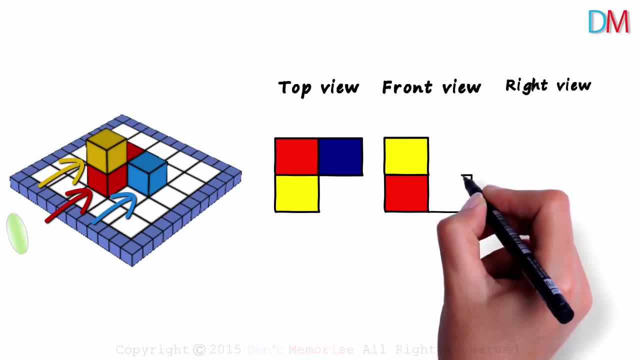 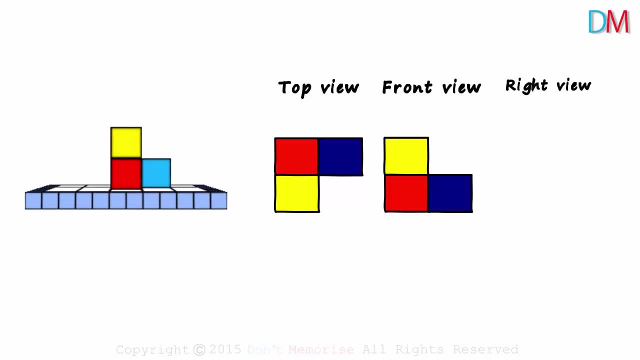 we will see the front face of the blue cube. We draw a blue square here, and that completes our front view. Let's rotate the figure to verify our answer. Yes, we are right. And what about the view from the right? In the same way, when we view the figure from the right, 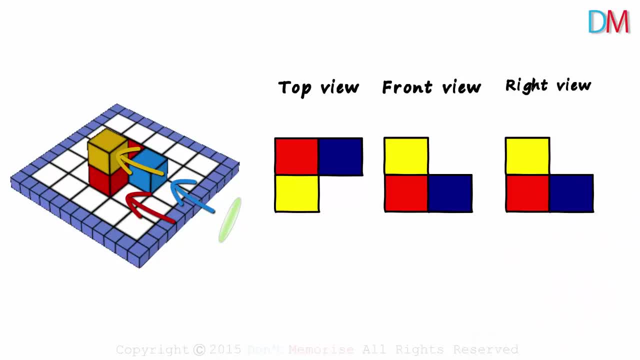 we will get a red, yellow and blue face like this. How will the view from the right look? This is the view from the right. Notice that the front view and the right view look the same. Drawing views from different angles simply requires a little bit of imagination. 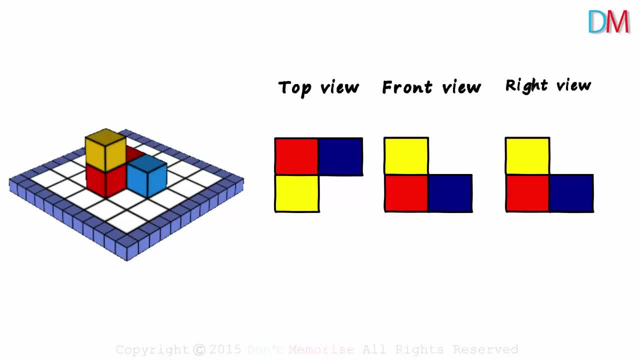 and with enough practice you will surely excel at it. 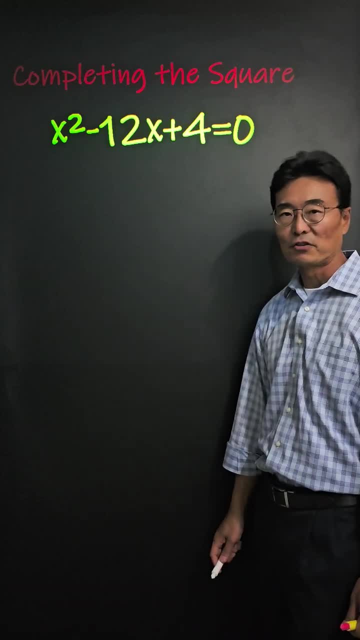 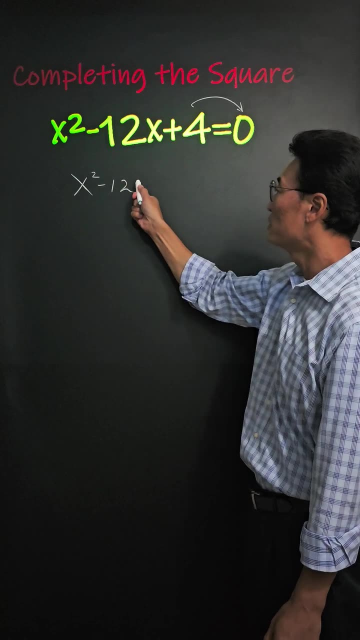 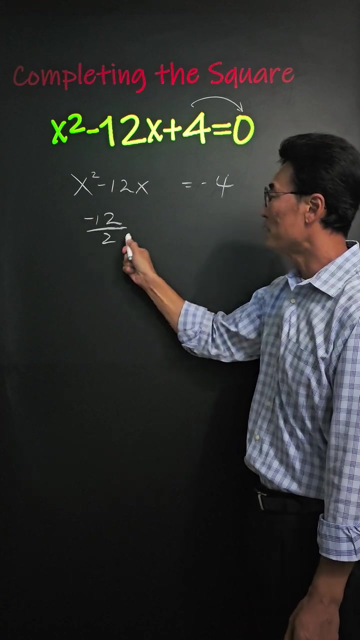 To solve for this equation I'm going to be using a method called completing the square. First bring the 4 over to the right side, giving us x squared minus 12x equals negative 4.. Then you take the coefficient of x, the negative 12 divided by 2, and then take that negative 6 and you square. 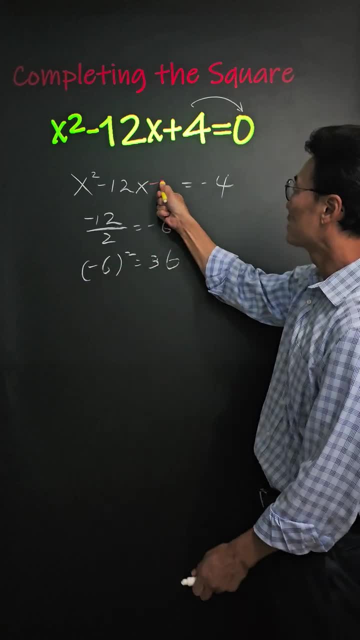 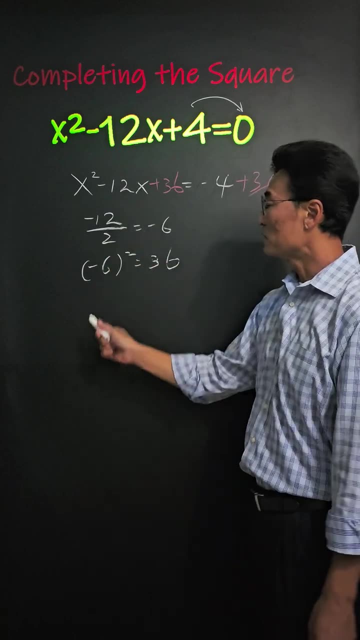 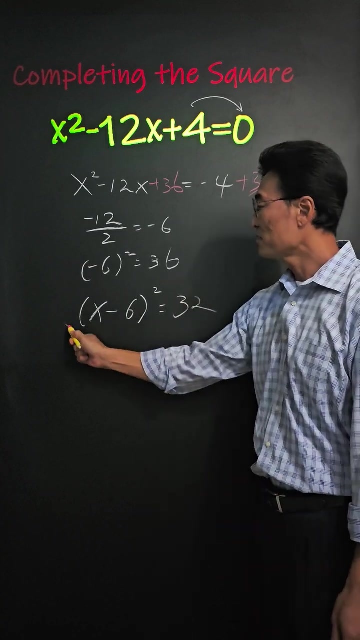 that and that's the number that we're going to add to the left side of the equation and the right side of the equation as well. If we factor the left side, we get x minus 6 squared The right side, we have a 32, and to solve for x we need to put in square root that to get rid of that square. 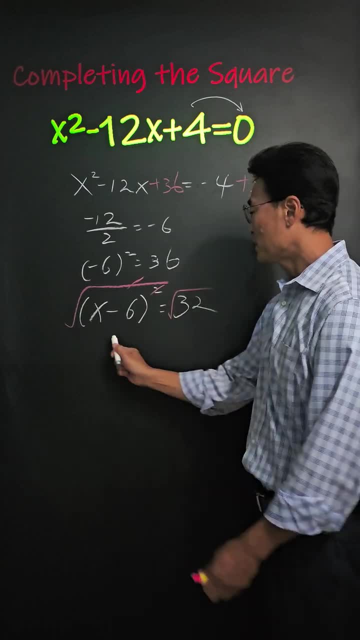 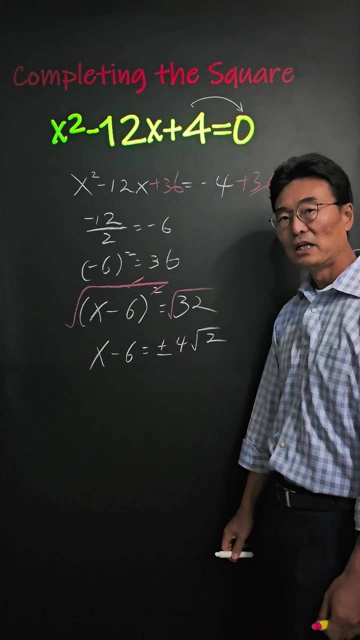 sign. and of course we have to do the same on the right side, giving us x minus 6 equals plus minus 4 root 2 if we simplify the root 32.. Finally, add the 6 so we get x equals 6 plus minus 4. 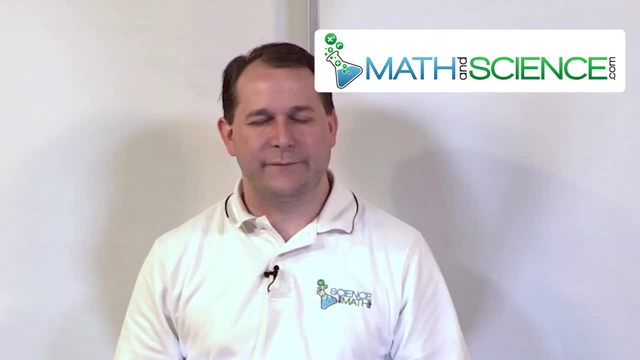 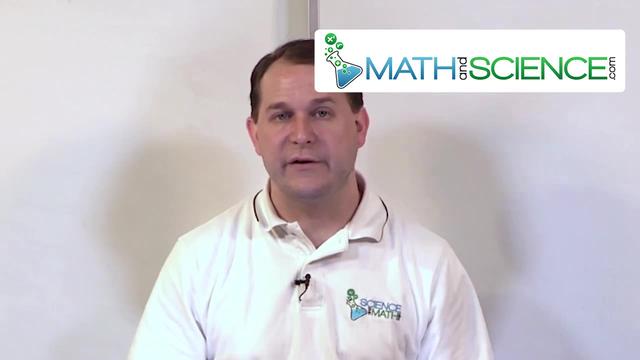 The z-score is going to be something that we're going to use constantly. Now it has a weird sounding name. A lot of students see the z-score. That must be hard, Really. it's just a weird name for something that's very, very simple to understand. Let me try to explain the z-score.